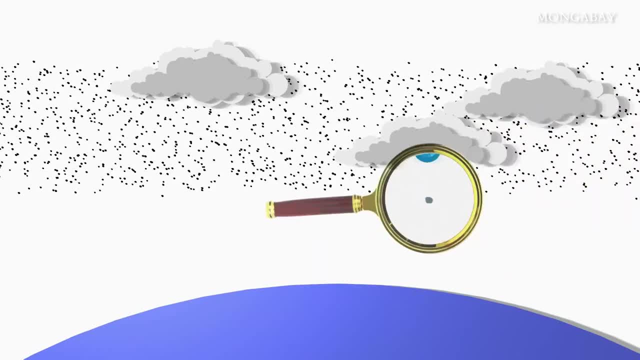 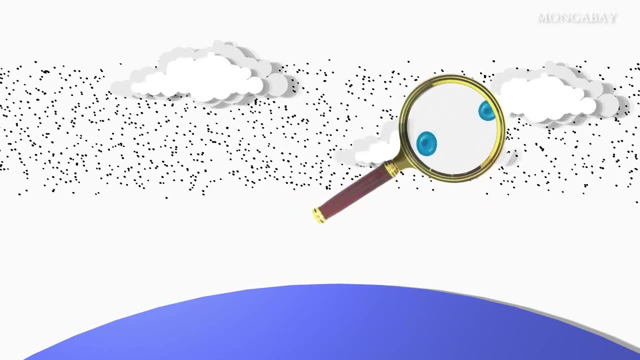 Aerosols can also make existing clouds more reflective. if particles move into a cloud, droplets tend to partially reform around them, leading to smaller droplets, which means greater surface area for the same amount of water. Greater surface area means greater scattering of light. This phenomenon is clearly visible. 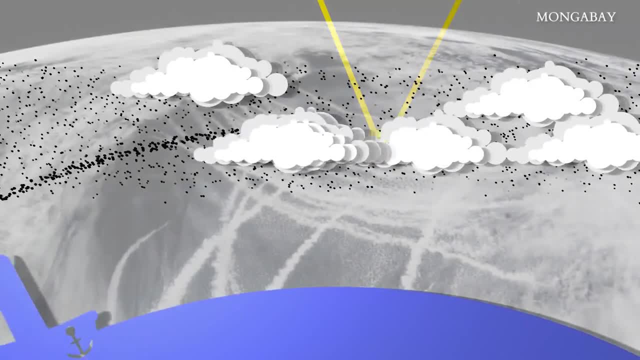 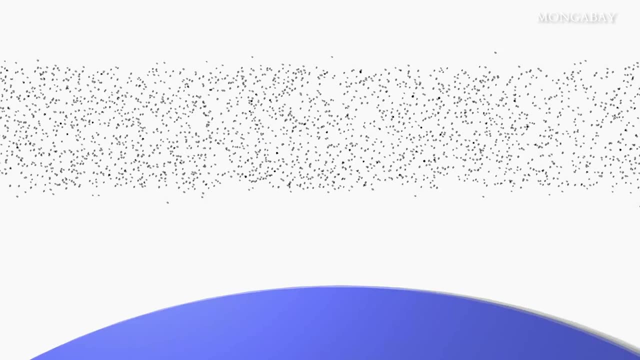 in satellite images of so-called ship tracks- bright lines where sulphate-spewing ships have passed. But not all aerosols are cooling Dark-coloured particles such as organic carbon and soot emitted by forest fires, brush clearing, wood charcoal and even dung-fired cooking stoves. 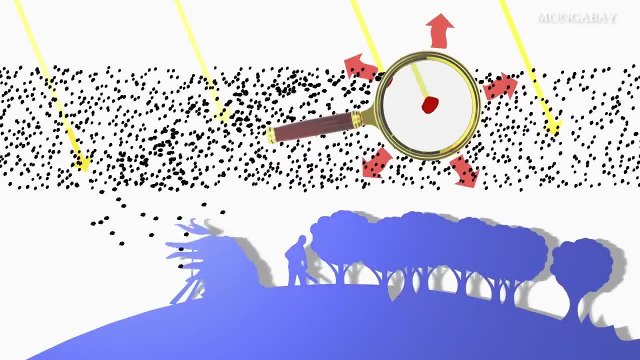 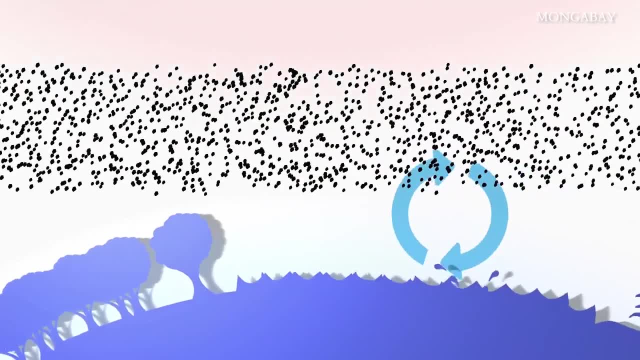 absorb light and re-radiate the energy around them as heat, warming the atmosphere while also cooling the surface. This effect can interfere with the water cycle by reducing the temperature gradient between Earth's surface and the atmosphere. This slows evaporation, which then 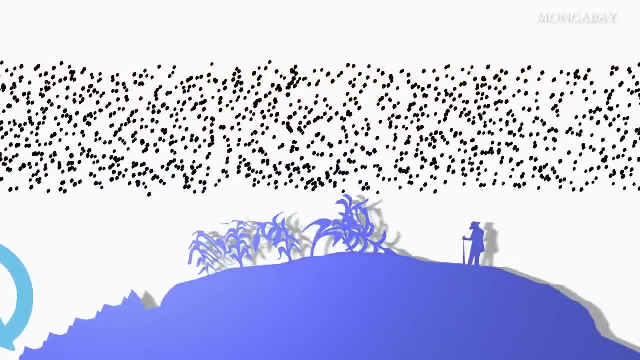 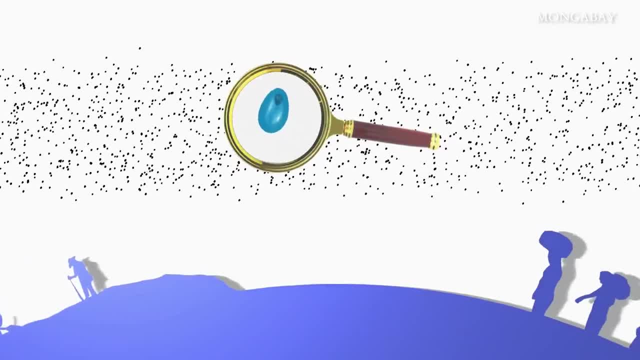 leads to less rain and sometimes drought. Another way aerosols reduce precipitation is when cloudwater droplets cling to the part of the planet. Another way aerosols reduce precipitation is when cloudwater droplets cling to the part of the planet. Another way aerosols reduce precipitation is when cloudwater droplets cling to the part of the planet. 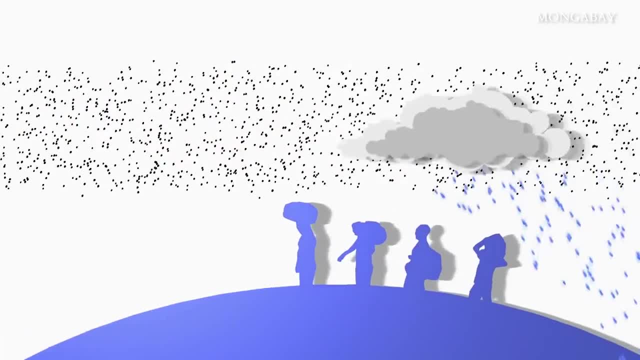 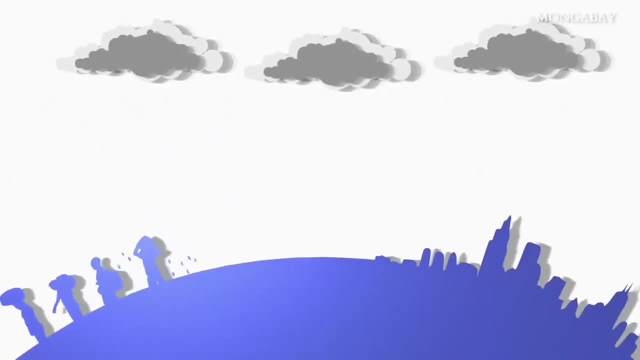 This might reduce rainfall at first, but it could also just delay it, leading to stronger rainfall elsewhere. Aerosols can even cause thunderstorms by holding onto droplets longer, allowing moisture-laden clouds to rise up higher in the atmosphere, forming thunderheads. 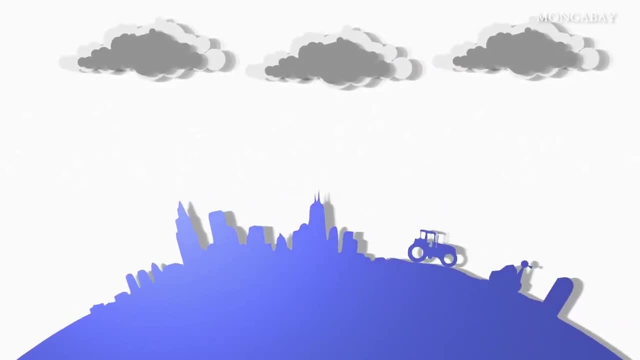 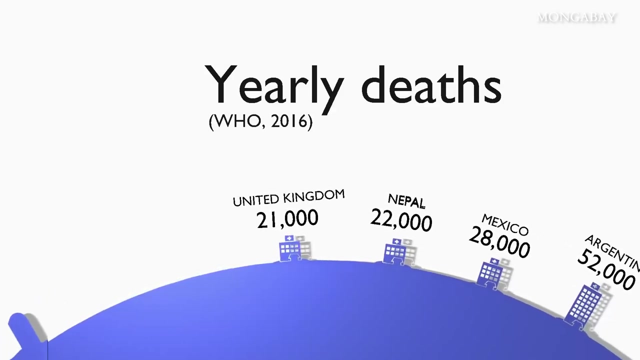 In the US, Midwest thunderstorms occur most often at mid-week, when urban pollutants are at their worst. Obviously, reducing human-produced aerosols is a good thing. Obviously, reducing human-produced aerosols is a good thing thing. Besides changing weather patterns, aerosols are blamed for the deaths of more than 6 million. 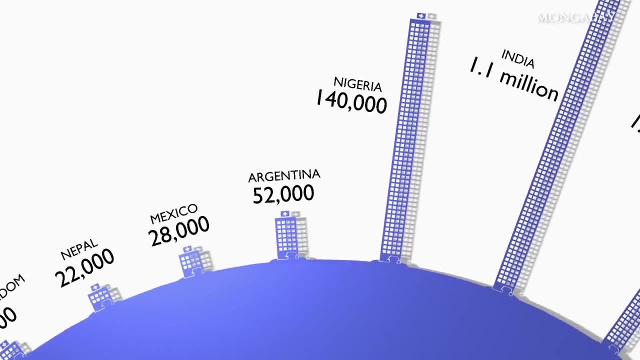 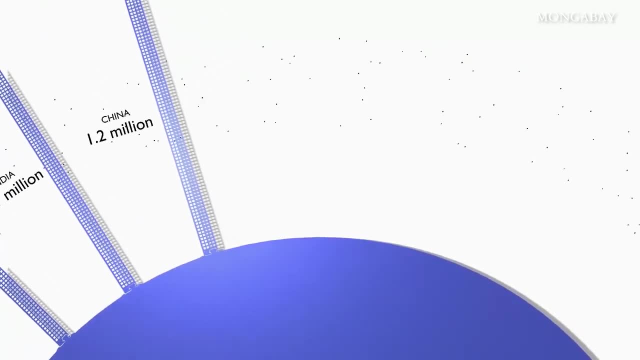 people every year. Fortunately, clean technologies have already helped reduce many aerosols, especially sulfate aerosols. But reducing them too fast is also a problem. That's because the cooling effect of aerosols offsets or masks some of the warming caused by greenhouse gases. 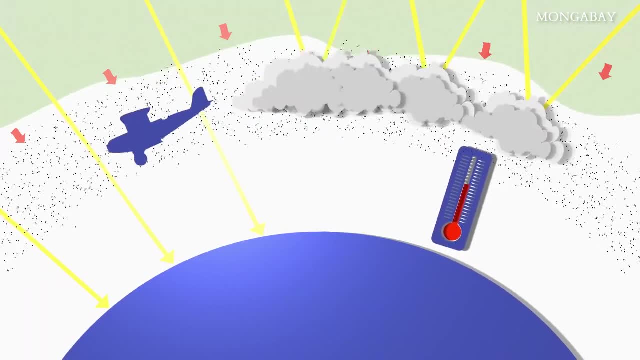 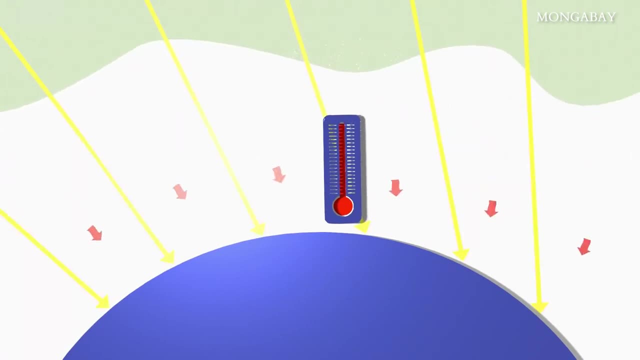 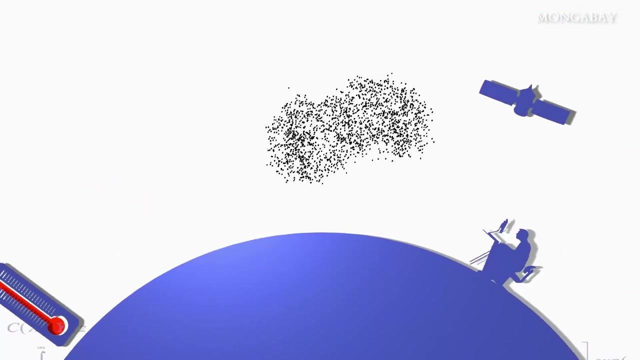 In fact, seeding clouds with aerosol particles has been proposed as a way to combat global warming. Meanwhile, some scientists warn that eliminating sulfate emissions could double global warming over the next 25 years. That figure isn't certain, however, because aerosols are still not well 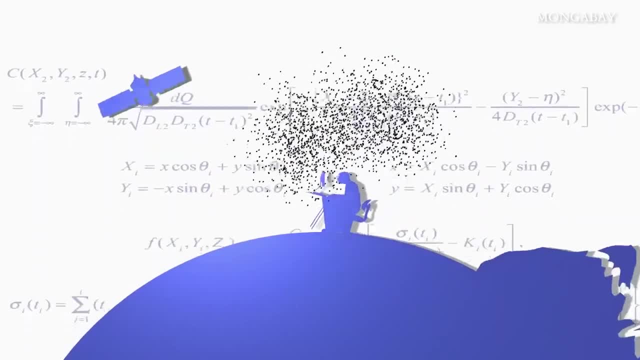 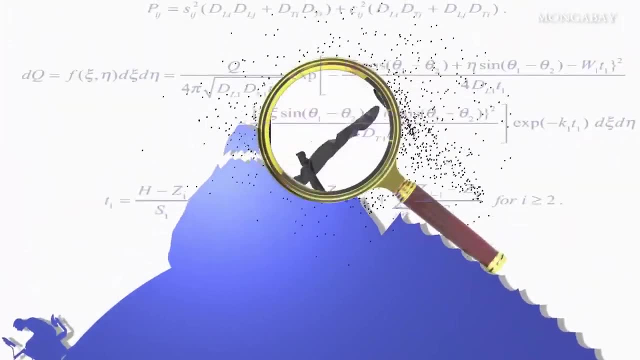 understood. They're hard to observe and hard to model with computers. Their effects depend on whether they're under clouds or on top of them, over land or over sea, or on a host of microscopic characteristics such as their size and shape. whether they adhere to other particles are in. 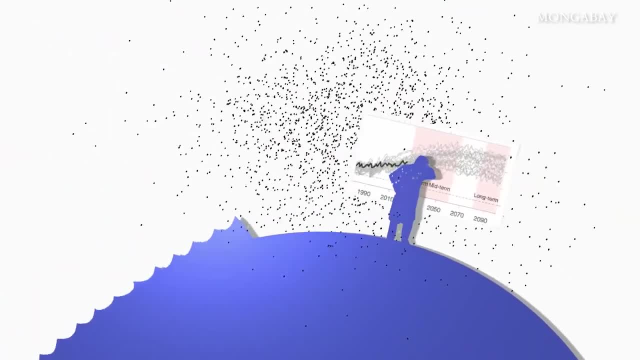 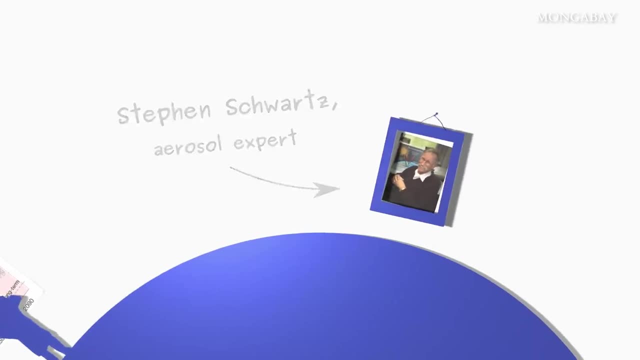 the presence of other particles or are in the presence of other particles. In fact, when it comes to predicting the climate, the effect of aerosols is still our largest source of uncertainty. That uncertainty has huge consequences when it comes to predicting the impacts of eliminating aerosols, says Stephen Schwartz, a climate scientist at the Brookhaven. 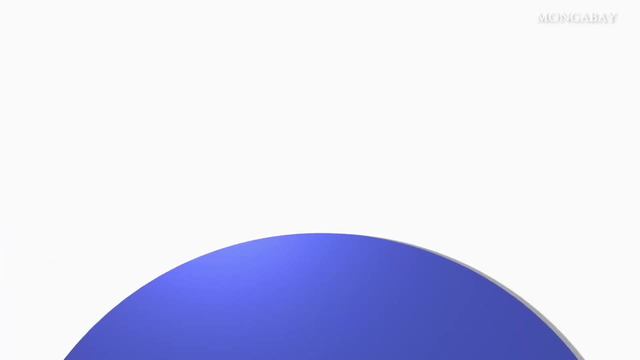 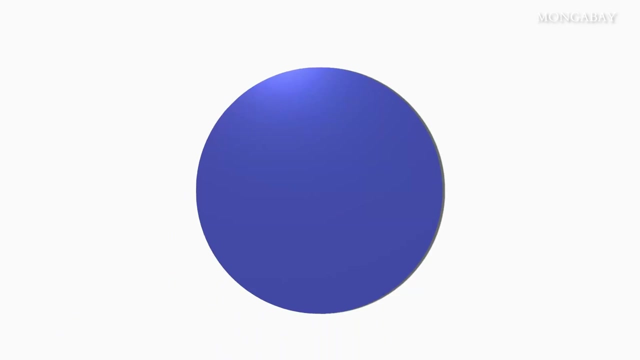 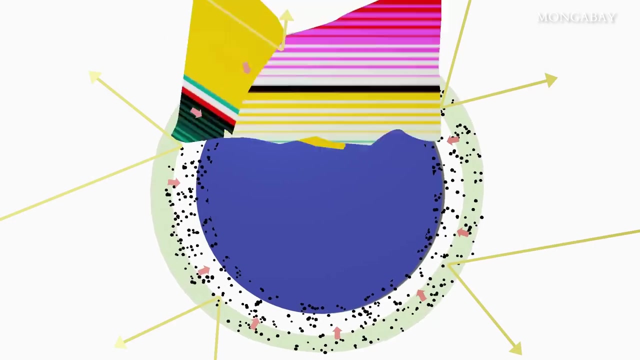 National Laboratory. That's because aerosols don't just mask global warming, they mask climate sensitivity. Climate sensitivity is a measure of how susceptible the Earth's current temperature is to changes in energy input. Greenhouse gases add energy, while aerosols typically subtract energy. Think of it like wrapping yourself in a blanket or applying an ice pack. 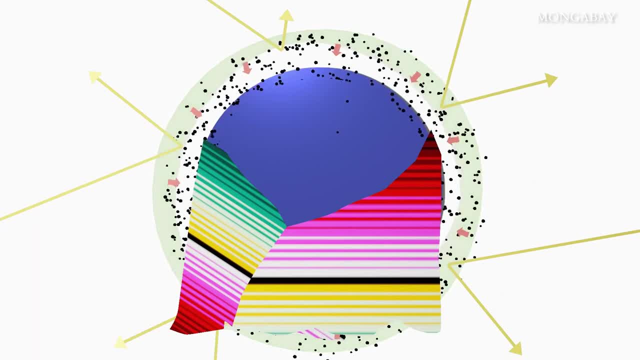 to your head. Climate sensitivity is like your metabolism. One blanket might be enough to warm others up, but you might still feel the cold. Unfortunately, we don't know how sensitive the Earth is. We do know how much Earth's temperature has risen in the last 150 years. That's been. 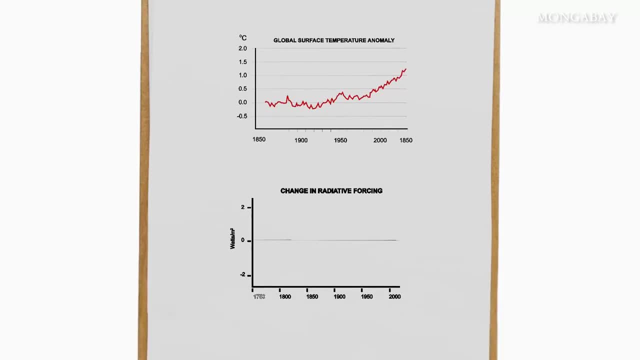 recorded. We also know how much greenhouse gases have increased the absorption of incoming solar radiation. The physics is well understood, But we don't know how much greenhouse gases have increased the absorption of incoming solar radiation. The physics is well understood, But we don't know how much. 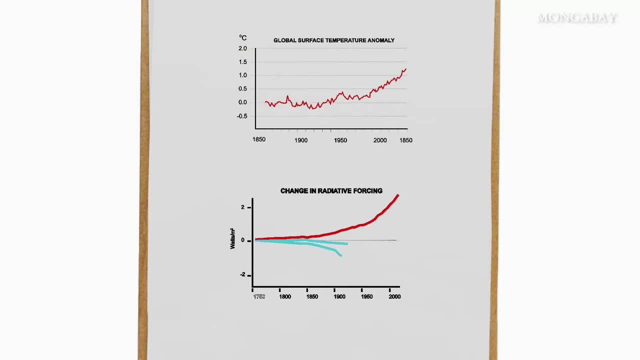 human-made aerosols are counteracting the heating effects of greenhouse gases, And that means we don't know the total change in energy. Aerosols might be cooling a lot or a little. As Schwartz points out, if aerosol cooling effects are minimal, then Earth's sensitivity to warming is low. 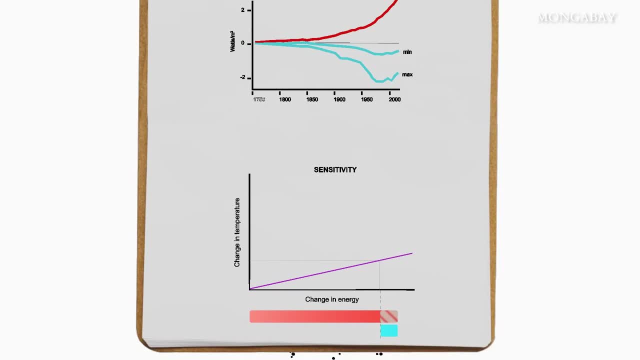 Eliminating aerosols would lead to only a relatively small change in temperature, But if aerosols are cooling a lot, then sensitivity must be high. That, he says, threatens us with a double whammy. If we manage to eliminate all aerosols, we're going to have a global warming crisis. 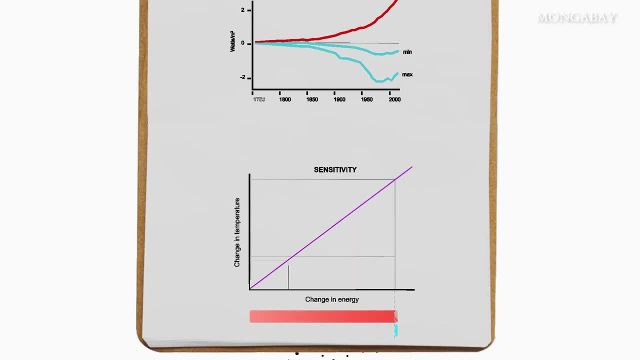 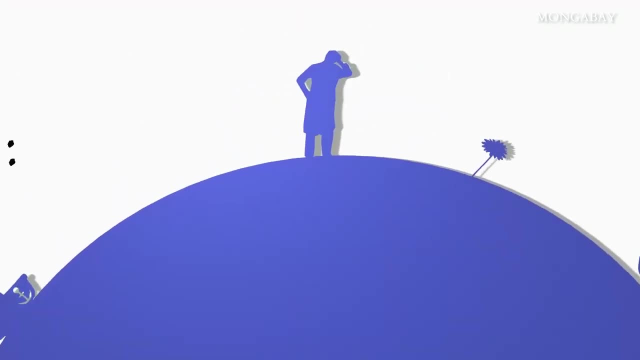 Not only might Earth's temperature go up, but it will go up faster due to Earth's higher sensitivity, And that would be bad for life on our planet. More study is urgently needed to know what human actions are best.